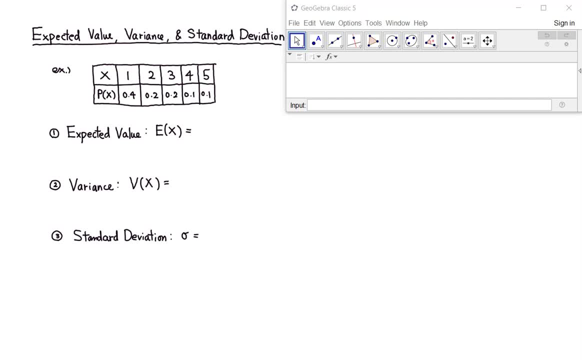 Alright, let's look at the expected value variance and the standard deviation. Alright, so it's probably the easiest to dive right into an example to demonstrate these things. Alright, so let's say you have a random variable and the possible values are 1,, 2, 3, 4, 5. And we listed each probability. So probability of getting a 1, x equals 1 is 0.4,, probability of 2 is 0.2, and so on. Alright, so the data is given. 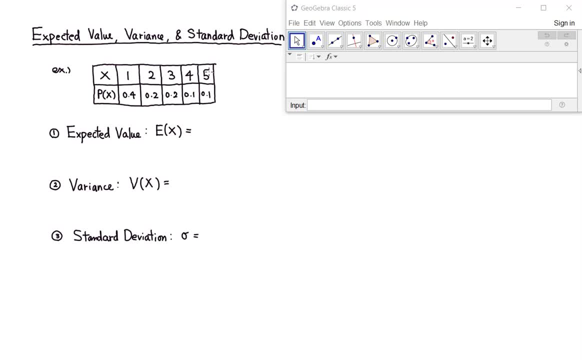 Alright, then we want to find the expected value of this random variable. Alright, expected value is essentially the weighed average. Alright, so what you do is, for this example, right so 1, right so 1 is the have the 0.4 probability of happening. 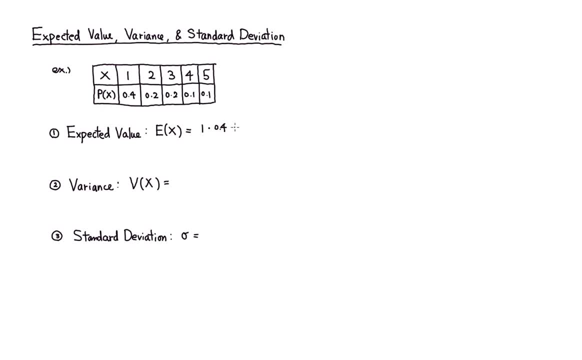 So you multiply 1 by 0.4, plus and 2 times its probability, so it's a 0.4.. So you multiply 1 by 0.2, and 3 times 0.2, plus 4 times 0.1, and plus 5 times 0.1.. 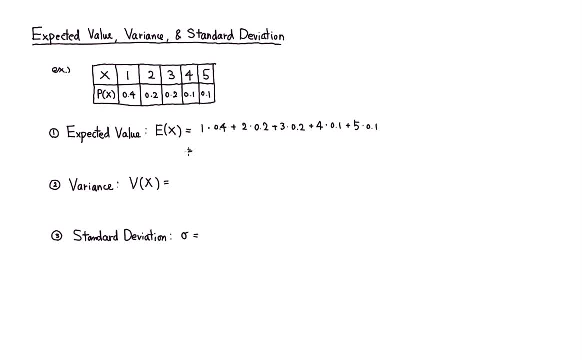 Then we just have to add them up, and I'm going to use a GeoGebra to compute it, Alright, so we're going to just type in, Actually do a little bit of mental computation too, Alright, 1 times 0.4 is 0.4.. 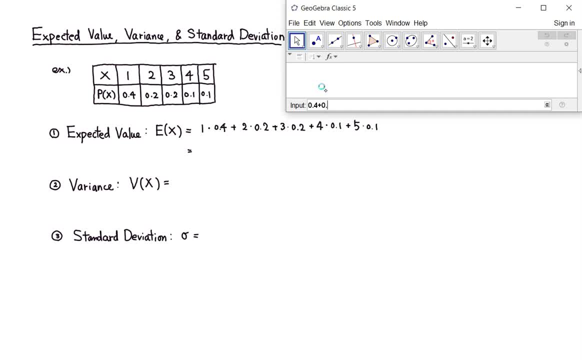 Alright, 2 times 0.2 is 0.4, again, And 3 times 0.2 is 0.6.. And 4 times 0.1 is 0.4.. Plus 5 times 0.1 is 0.5.. 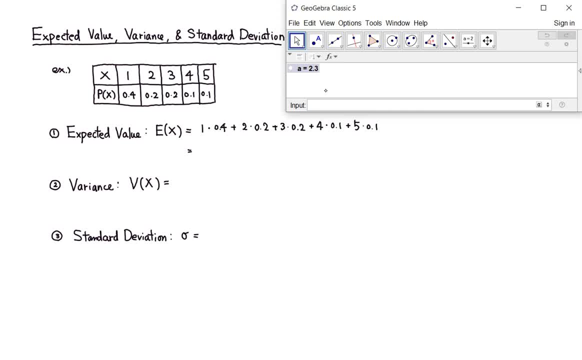 Alright. so hit enter Alright, so it's a 2.3.. So expected value is 2.3.. Alright, so we got that Alright. so that's how you find the expected value. Alright, variance is expected value of the square difference from the mean. 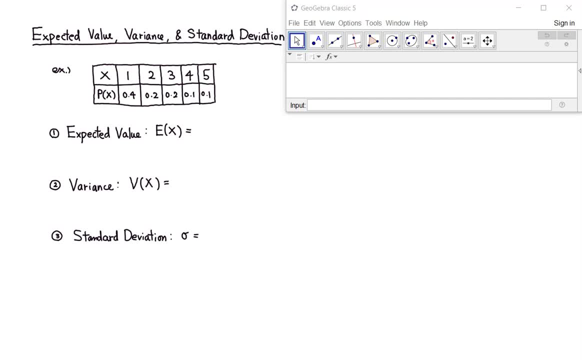 Alright, let's look at the expected value variance and the standard deviation. Alright, so it's probably the easiest to dive right into an example to demonstrate these things. Alright, so let's say you have a random variable and the possible values are 1,, 2, 3, 4, 5. And we listed each probability. So probability of getting a 1, x equals 1 is 0.4,, probability of 2 is 0.2, and so on. Alright, so the data is given. 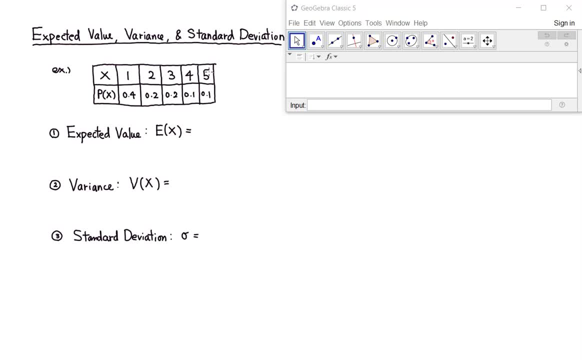 Alright, then we want to find the expected value of this random variable. Alright, expected value is essentially the weighed average. Alright, so what you do is, for this example, right so 1, right so 1 is the have the 0.4 probability of happening. 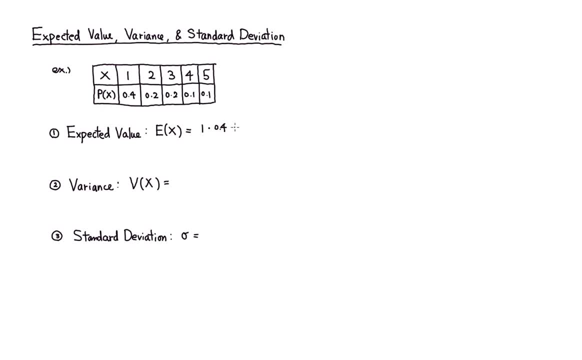 So you multiply 1 by 0.4, plus and 2 times its probability, so it's a 0.4.. So you multiply 1 by 0.2, and 3 times 0.2, plus 4 times 0.1, and plus 5 times 0.1.. 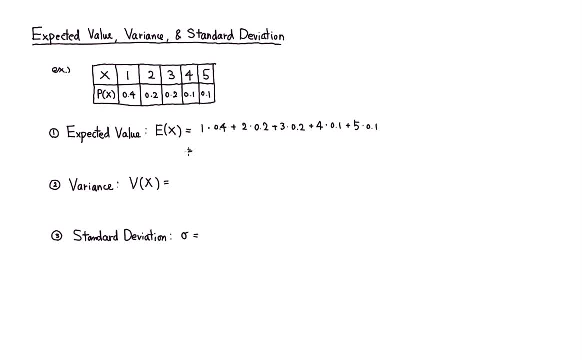 Then we just have to add them up, and I'm going to use a GeoGebra to compute it, Alright, so we're going to just type in, Actually do a little bit of mental computation too, Alright, 1 times 0.4 is 0.4.. 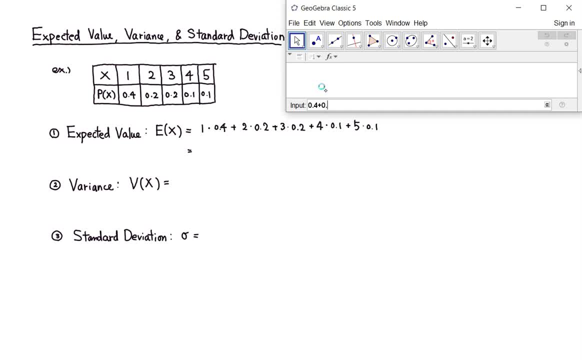 Alright, 2 times 0.2 is 0.4, again, And 3 times 0.2 is 0.6.. And 4 times 0.1 is 0.4.. Plus 5 times 0.1 is 0.5.. 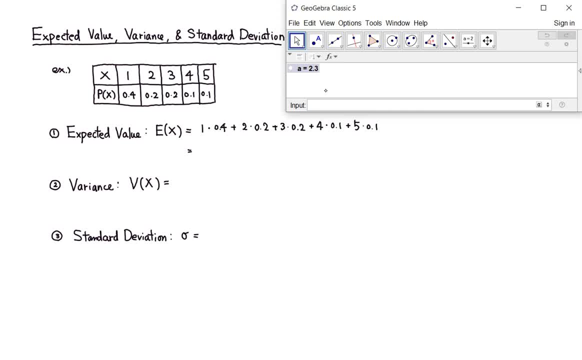 Alright. so hit enter Alright, so it's a 2.3.. So expected value is 2.3.. Alright, so we got that Alright. so that's how you find the expected value. Alright, variance is expected value of the square difference from the mean. 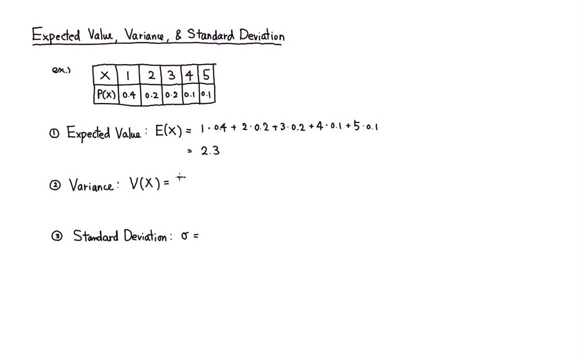 So if you write it in terms of expected value, so this is expected value of the square difference. So we take the difference, So we take the difference between the x value, random variable value, then minus the expected value, So it's going to be 2.3.. 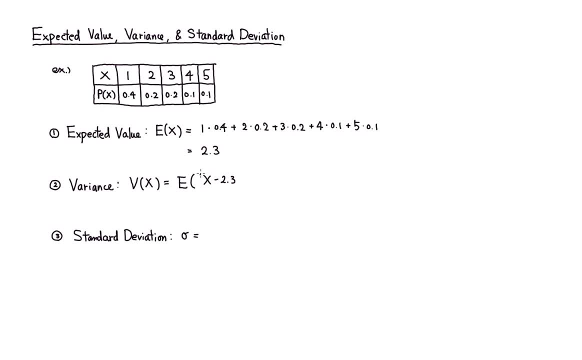 Alright, And then you square that Alright. Alright, so maybe we should make a list. So here: Alright, so I'm going to make a list of square difference. Alright, so the square difference would be: I'm going to just do x minus expected value, 2.3, then square that. 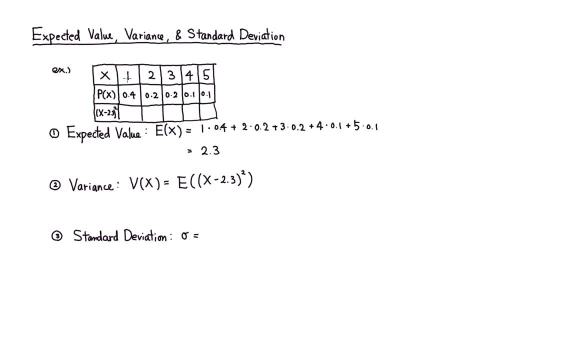 Alright, So here. Alright. so 1 minus 2 minus 2.3 is 1.3.. So it's going to be 1.3 squared Alright. Alright, it's. let's see. 2 minus 2.3 is negative 0.3 squared. 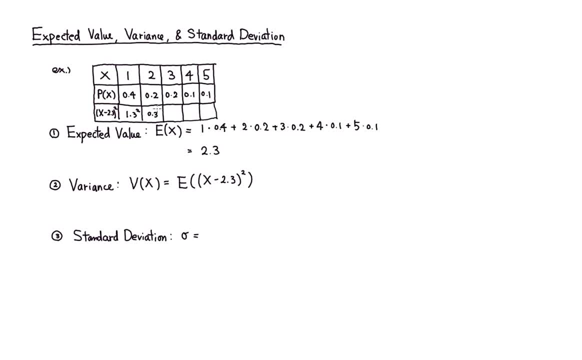 So I'm going to just say 0.3 squared, Because negative is not going to matter, because it gets squared anyway. Alright, so it's. let's see: 3 minus 2.3 is 0.7.. So I'm going to just say 0.7 squared. 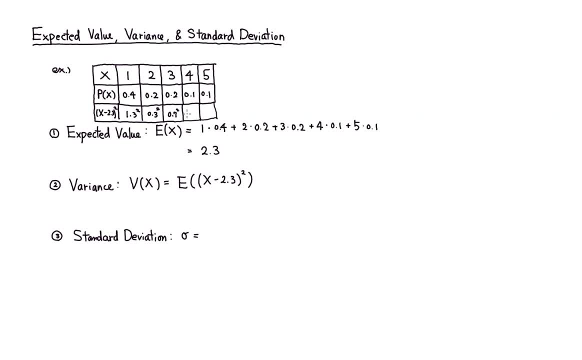 Alright, And 4 minus 2.3 is 1.7.. Then you have to square that, And 5 minus 2.3 is 2.7. And square that. Alright, Then you just need to find its expected value. 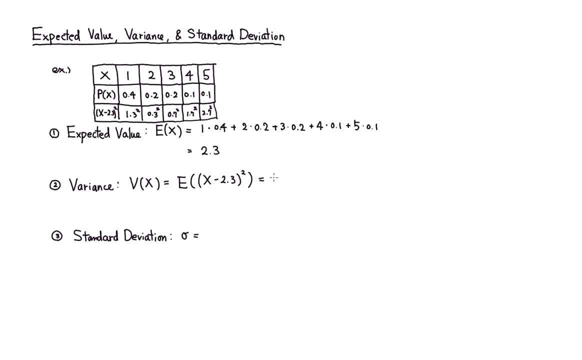 So all you have to do is Alright. So value is 1.3 squared, But the problem Probability is 0.4.. Alright, Then you have 0.3 squared. Probability is 0.2.. 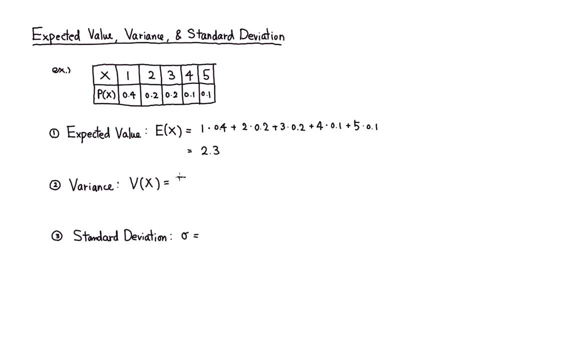 So if you write it in terms of expected value, so this is expected value of the square difference. So we take the difference, So we take the difference, So we take the difference between the x value, random variable value, then minus the expected value. 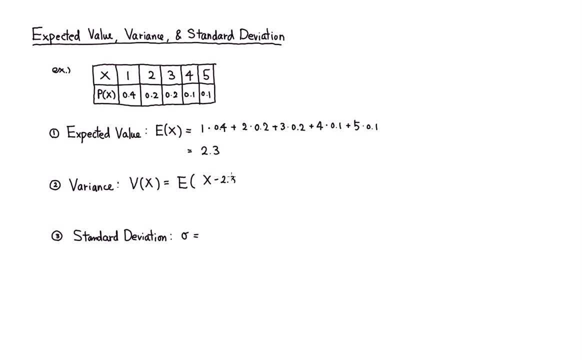 So it's going to be 2.3.. Alright, and then you square that. Alright, so maybe we should make a list. So here, Alright, so I'm going to make a list of square difference. Alright, so the square difference would be: I'm going to just do x minus expected value, 2.3, then square that. 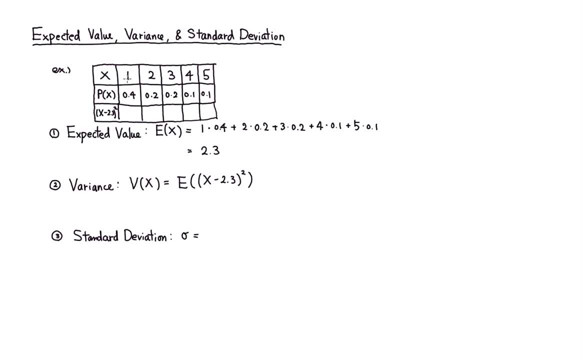 Alright, so here. Alright, so 1 minus 2.3.. Alright, so 1 minus 2.3.. Alright, so 1 minus 2.3 is 1.3.. So it's going to be 1.3 squared. 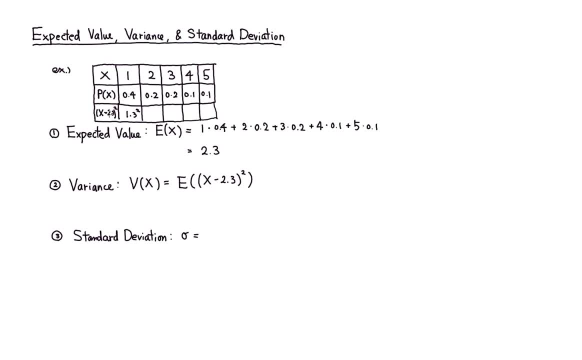 Alright, Alright it's. let's see: 2 minus 2.3 is negative, 0.3 squared. So I'm going to just say 0.3 squared, because negative is not going to matter, because it gets squared anyway. 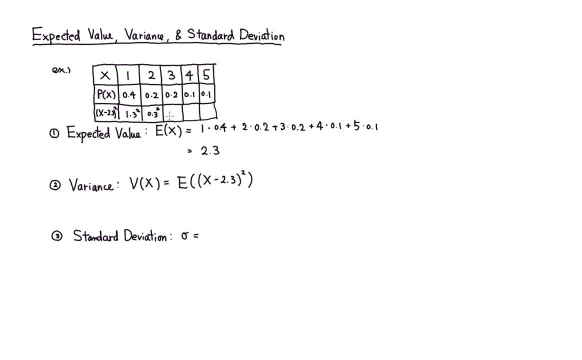 Alright, so it's. let's see: 3 minus 2.3 is 0.7.. So I'm going to just say 0.3 squared right, And 4 minus 2.3 is 1.7.. 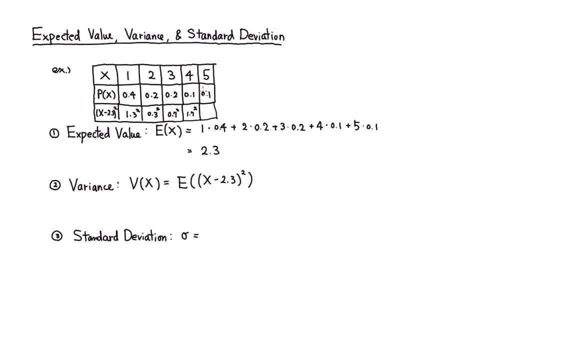 Then you have to square that, And 5 minus 2.3 is 2.7.. And square that, Alright. then you just need to find its expected value. So all you have to do is right. So value is 1.3 squared. 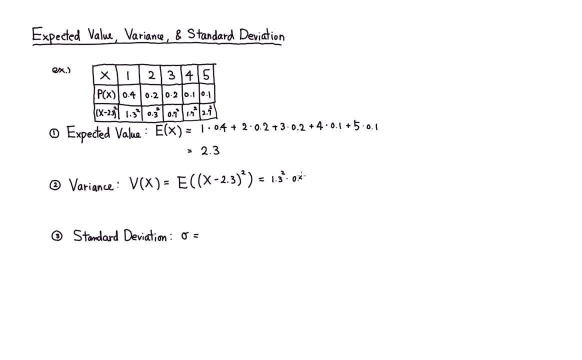 But the product, But the probability is 0.4.. Alright, then you have 0.3 squared. Probability is 0.2.. Plus 0.7 squared Times. probability is 0.2, again Plus 1.7 squared. 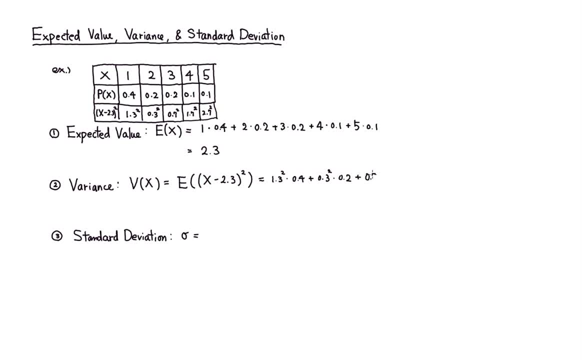 Plus 0.7 squared Times, probability is 0.2. again Plus 1.7 squared, And then probability is 0.1.. And the last one is 2.7 squared And the probability is 0.1.. 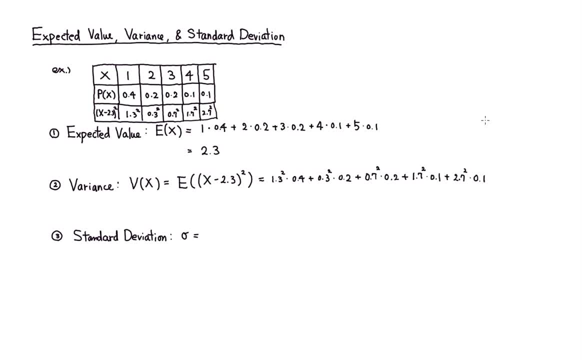 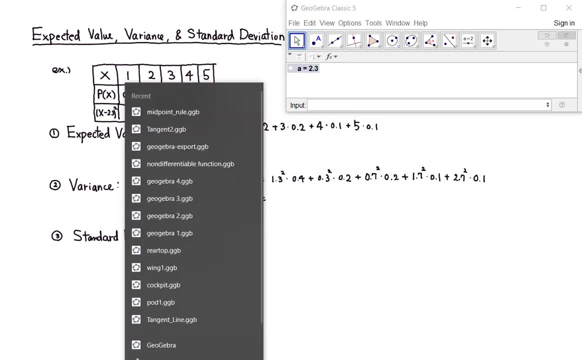 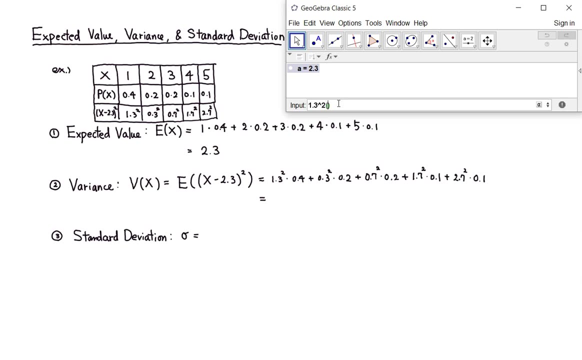 Alright, So exactly the same way. So it's the expected value of the squared difference from the mean. Alright, Then let's compute this value. Alright, So we have 1.3 squared times 0.4.. 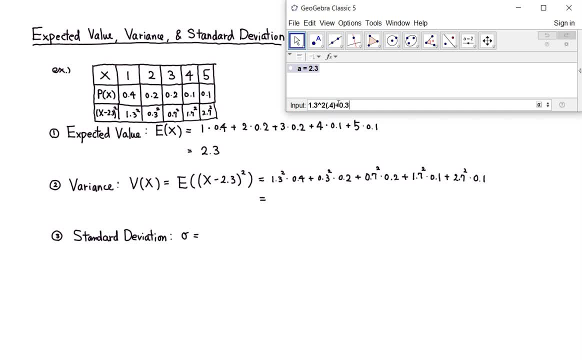 Plus 0.4.. So we have 0.3 squared times 0.2.. Alright, I guess maybe I'll just stop writing 0.. Plus 0.4 squared times 0.2.. Plus 1.7 squared times 0.1.. 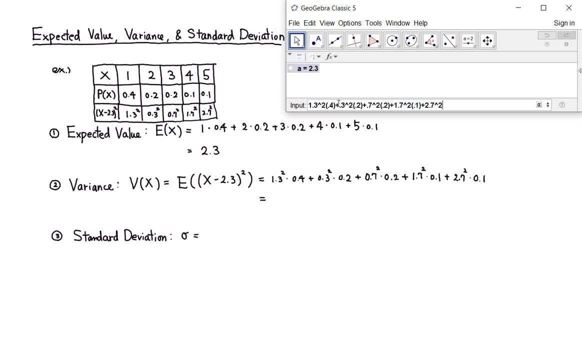 Plus 2.7 squared Times, 0.1.. Alright. Then hit enter Alright, So it came out to be 1.81.. So 1.81 is the variance, Alright, And variance is actually the square of the standard deviation. 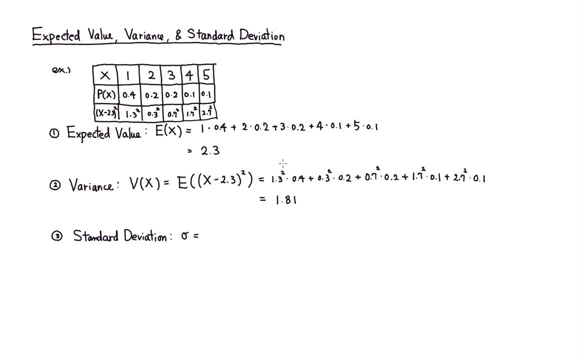 So if you want to find the standard deviation, all you have to do is So. this is actually the same thing as standard deviation, squared Alright, Then expect: Let's see So here. So square root of the variance. 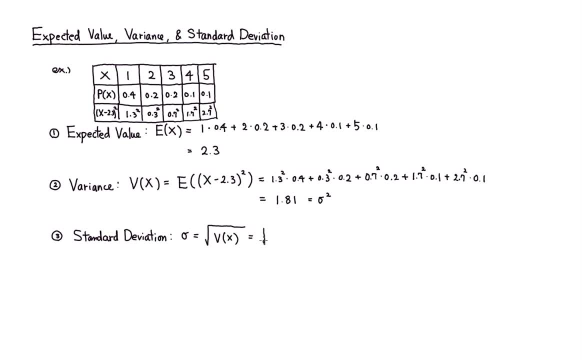 Alright, So this is just going to be a square root, of Which we have 1.81.. And what number is that? So you have a square root of 1.81.. Which come out to be 0.35.. 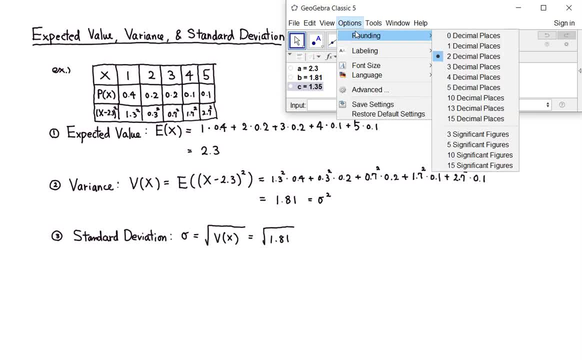 Is that an exact value? Let's see, I'm going to just change the rounding and see if it's Okay, It's not the exact value, But so this is about Here. Let's see: Oops, 0.. 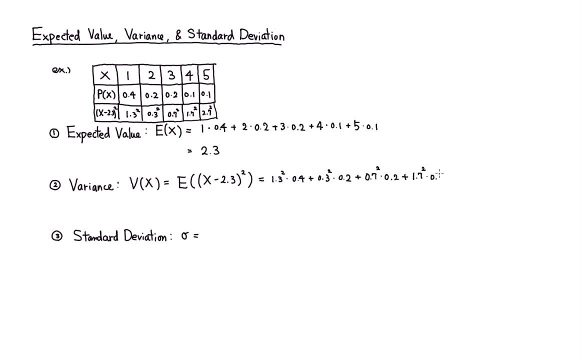 And then probability is 0.1.. And the last one is 2.7 squared And the probability is 0.1.. Alright, so exactly the same way. So it's the expected value of the squared difference from the mean. 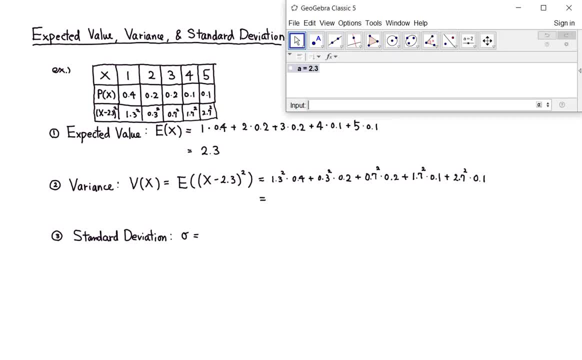 Alright, then let's compute this value. Alright, So we have 1.3 squared times 0.4.. Plus 0.3 squared times 0.2.. Alright, I guess. maybe I'll just stop writing 0.. 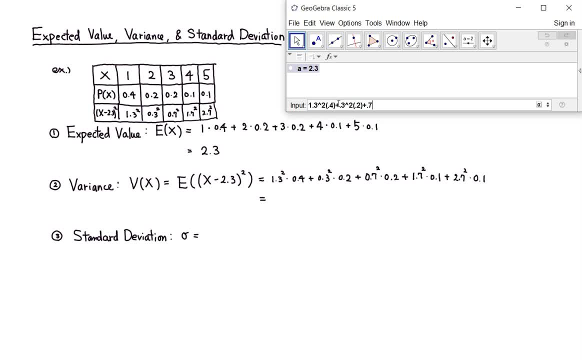 Plus 0.4 squared times 0.2.. Plus 1.7 squared times 0.1.. Plus 2.2.. Plus 1.7 squared times 0.1.. Alright, Then hit enter. Alright, So it came out to be 1.81.. 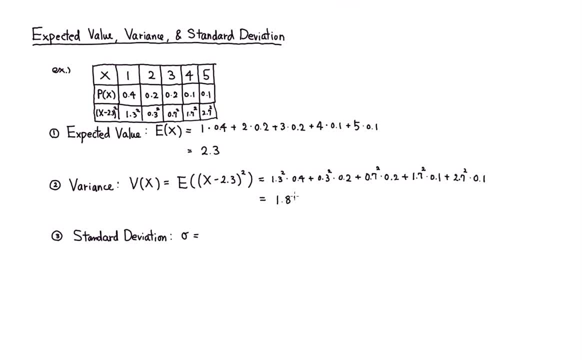 So 1.81 is the variance, Alright, And variance is actually the square of the standard deviation. So if you want to find the standard deviation, all you have to do. So this is actually the same thing as standard deviation squared. 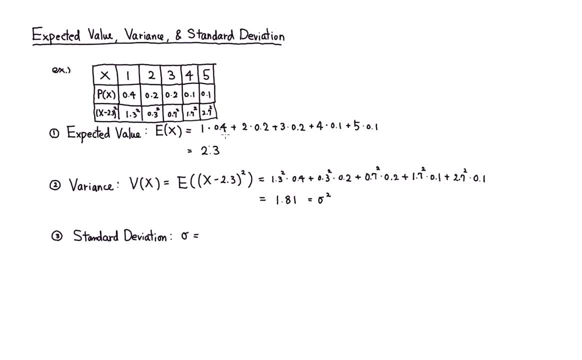 Alright, Then expected value. Let's see So here. So square root of the variance, Alright, So this is just going to be a square root of Which we have 1.81.. And what number is that? 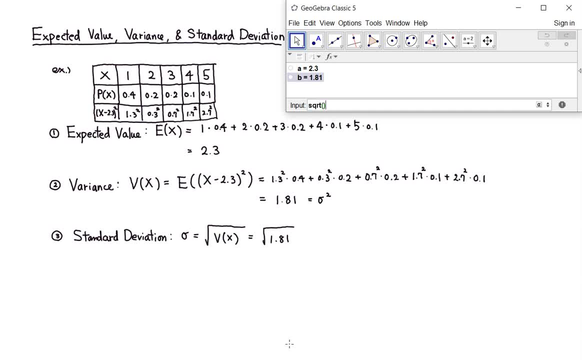 So you have a square root of 1.81.. Which come out to be 0.35.. Is that an exact value? Let's see. I'm going to just change the rounding and see if it's Okay. It's not the exact value. 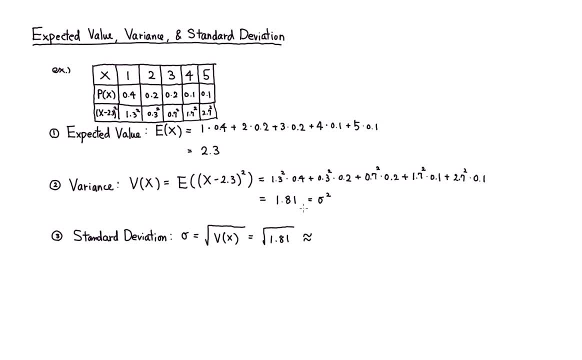 So this is about Here. Let's see: Oops, 0.. 1 point. I'll just say 1.35.. About 1.35.. Alright, So that's the standard deviation of this data set, Alright.